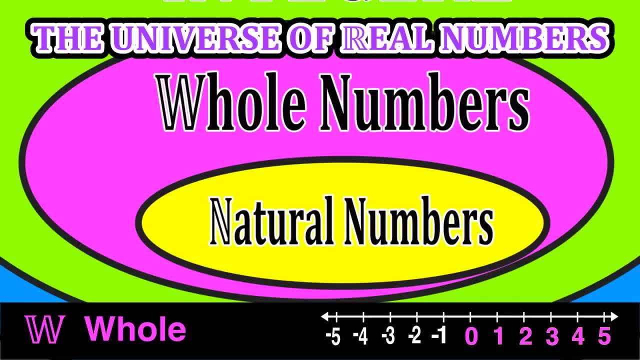 three, four, five and anything else, going on and on and on in a positive direction, but it's starting at zero, whereas the natural numbers start at one. Now, the whole numbers are a smaller subset of the entire set of numbers, which is equal to one, two, three, four, five, four, six, seven. 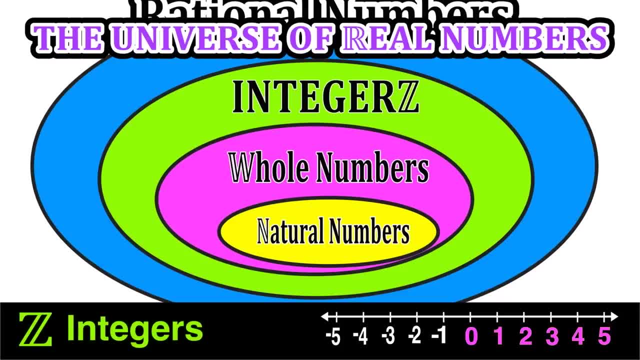 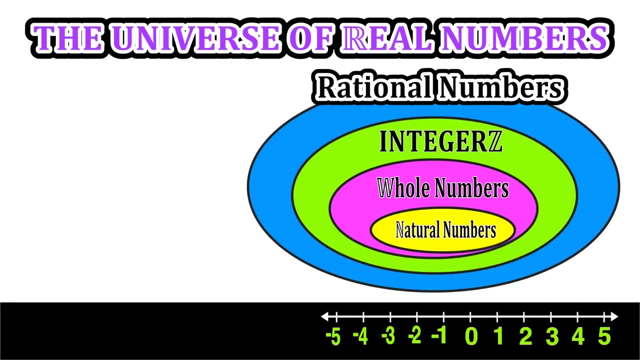 integers. Now what integers are? all of the natural numbers and zeros, so all of the whole numbers as well, and their negative counterparts. So now we move on forever in a positive direction and a negative direction here, And all of these are subsets of the greater universe of rational. 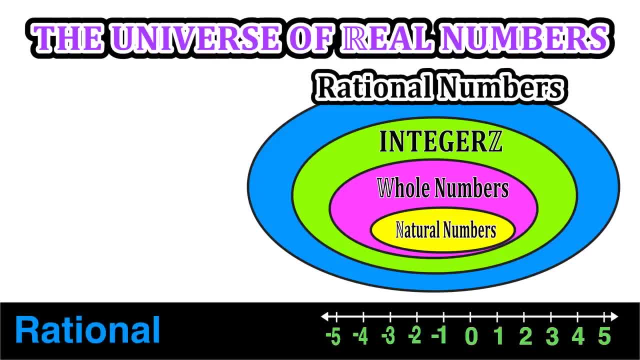 numbers. Now the rational numbers will fill in the gaps in between those integers on the number line, In this case any number that can be written as a fraction a over b, where a and b are both whole numbers here, And an example would be one half. Now this does not actually cover every. 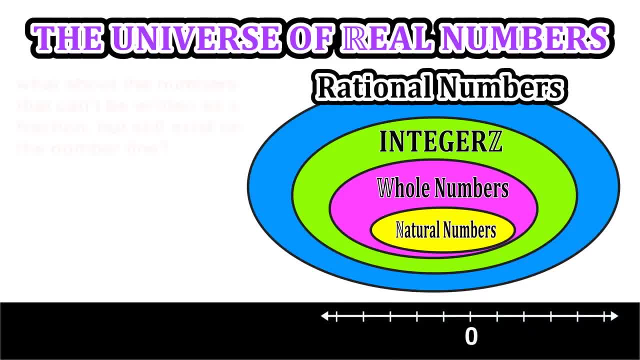 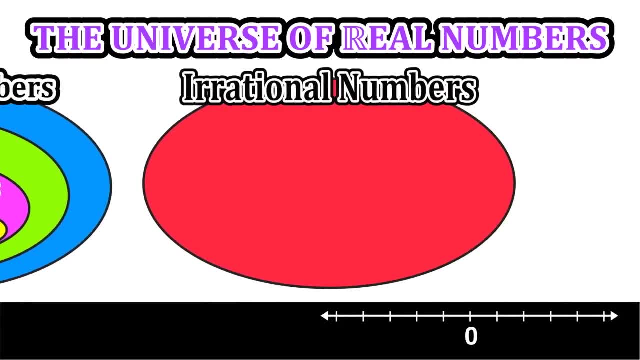 possible value that can be found on the number line. We can ask ourselves, what about the numbers that can't be written as a fraction? And what about the numbers that can't be written as a fraction but still exist on that number line? This would be the set of irrational numbers, And 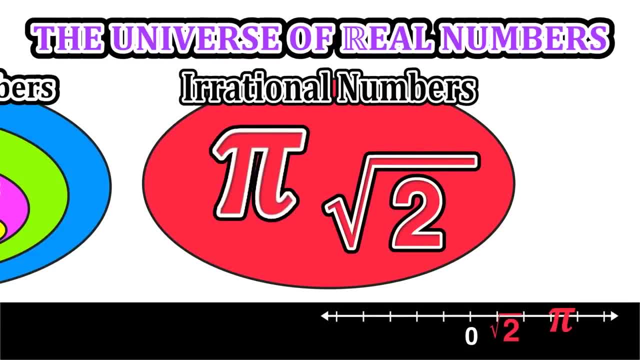 examples would include pi and the square root of two, since two is not a perfect square. Such irrational numbers do exist on the number line. However, they cannot be written as a fraction, the way that a rational number can be. Now we notice that there is no overlap between the rational. 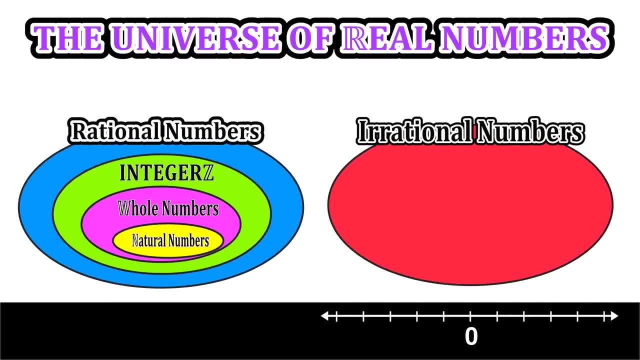 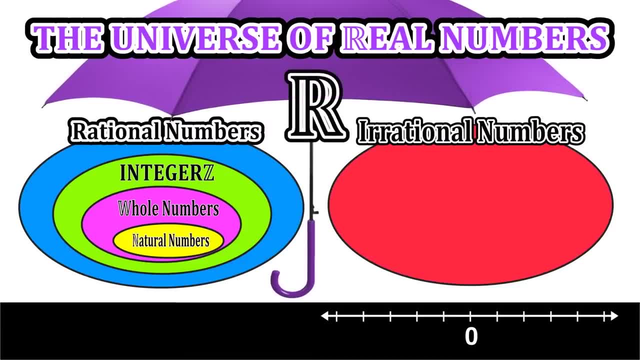 numbers and irrational numbers, since no number can be both rational and irrational at the same time. And both of these sets of numbers are covered under the umbrella of the real numbers. So a real number is anything that can be found on that number line. And visualizing this universe of real numbers, 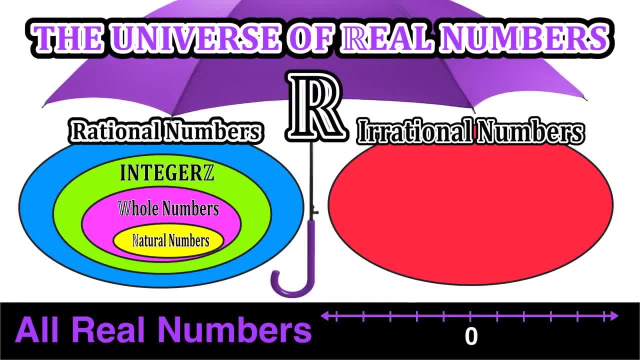 should really help us to understand when we see that phrase. all real numbers. Keep this in mind moving forward, and I'll make things much easier for you. And don't those colors look nice? See ya, Thanks guys for checking out that lesson and go ahead and. 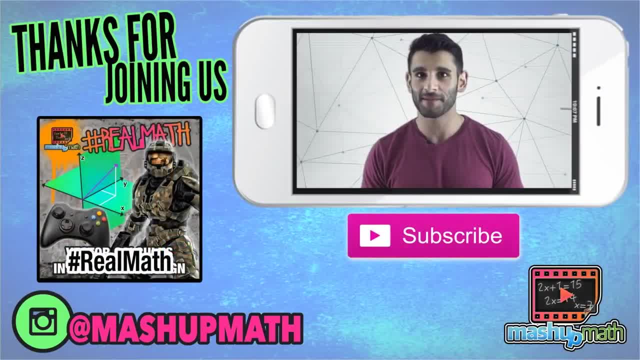 follow us on Instagram at mashupmap. It's a pretty cool Instagram account. I promise you Take a look. 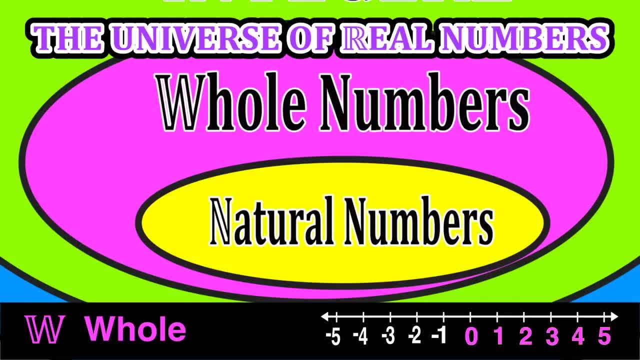 five and anything else, going on and on, and on in a positive direction, but it's starting at zero, whereas the natural numbers start at one. Now, the whole numbers are a smaller subset of the natural numbers, And so what happens if you add one to one of the natural numbers? 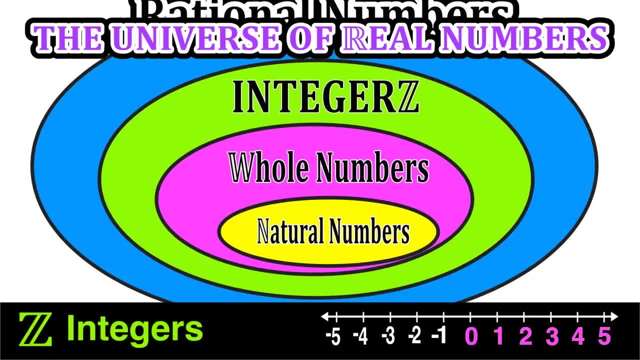 We start with one, and then two, and then four, and then six integers. Now what integers are? all of the natural numbers and zeros, so all of the whole numbers as well, and their negative counterparts. So now we move on forever in a positive direction and a. 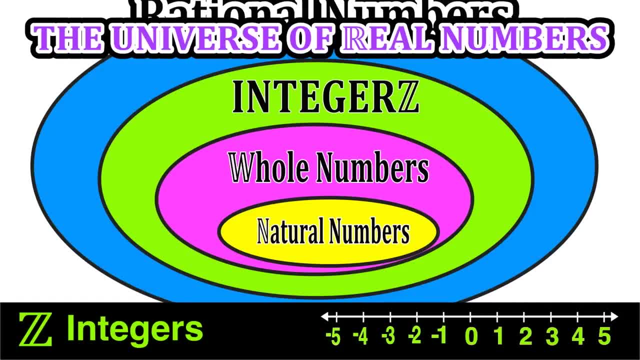 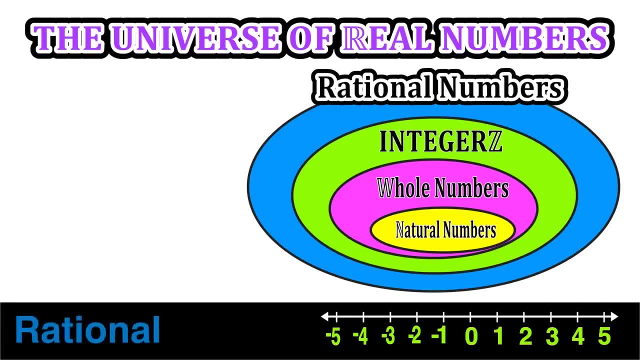 negative direction here. And all of these are subsets of the greater universe of rational numbers. Now the rational numbers will fill in the gaps in between those integers on the number line, In this case any number that can be written as a fraction, a over b, where a and b are both. 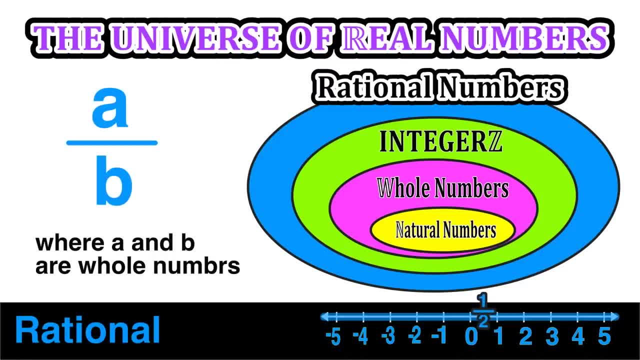 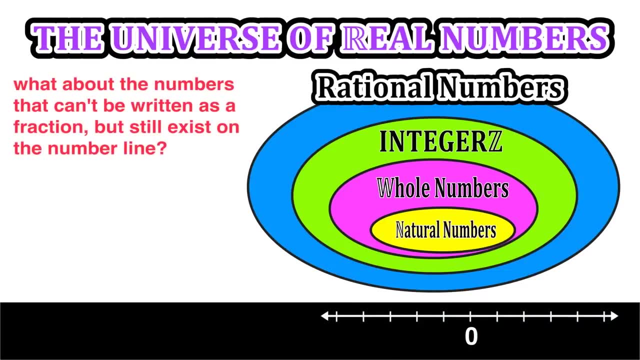 whole numbers here, And an example would be one half. Now this does not actually cover every possible value that can be found on the number line. We can ask ourselves: what about the numbers that can't be written as a fraction, And what about the numbers that can't be written as a? 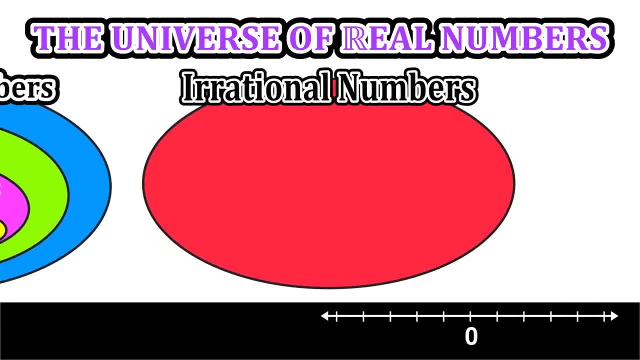 fraction, but still exist on that number line. This would be the set of irrational numbers, And examples would include pi and the square root of two. since two is not a perfect square, Such irrational numbers do exist on the number line. However, they cannot be written as a fraction. the 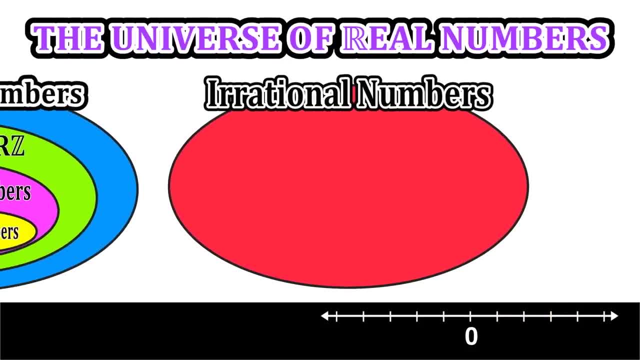 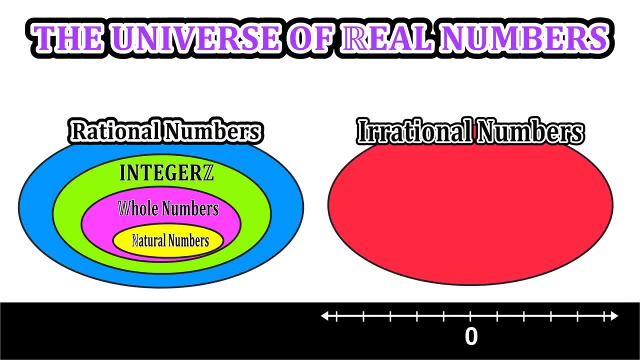 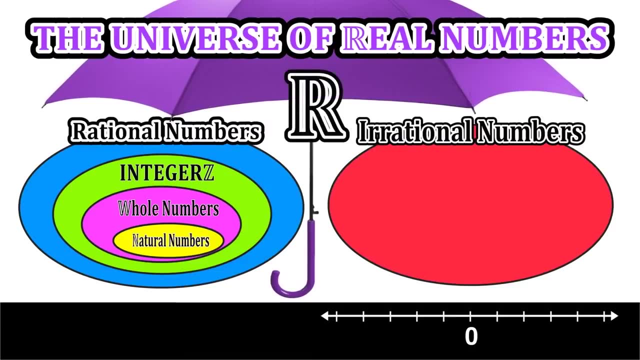 way that a rational number can be. Now we notice that there is no overlap between the rational numbers and irrational numbers, since no number can be both rational and irrational at the same time, And both of these sets of numbers are covered under the umbrella of the real numbers. So a real number. 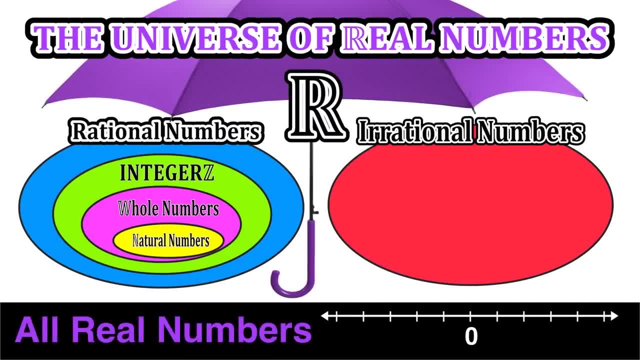 is anything that can be found on that number line, And visualizing this universe of real numbers should really help us to understand when we see that phrase: all real numbers. Keep this in mind moving forward and I'll make things much easier for you. And don't those colors look nice, See ya? 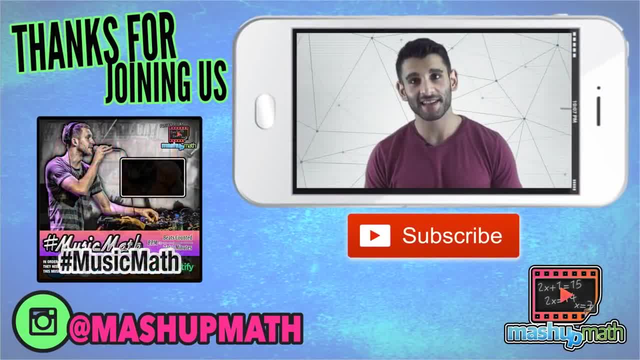 Thanks, guys for checking out that lesson and go ahead and follow us on Instagram at mashupmap. It's a pretty cool Instagram account. I promise you Take a look.